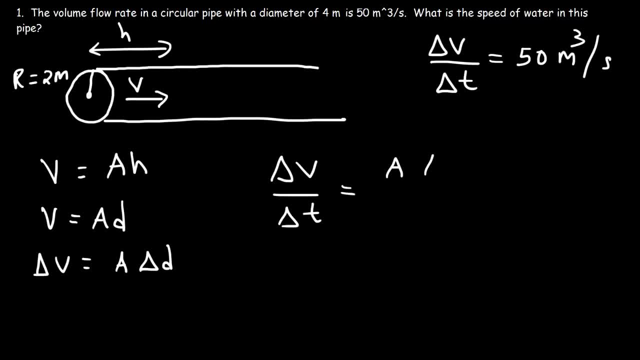 delta T, that's going to be A times the displacement divided by the time. Displacement over time is velocity, So the volume flow rate is equal to the cross-sectional area times the speed of water. So we have a volume flow rate of 50 cubic meters per second And the cross-sectional area is pi? r squared. 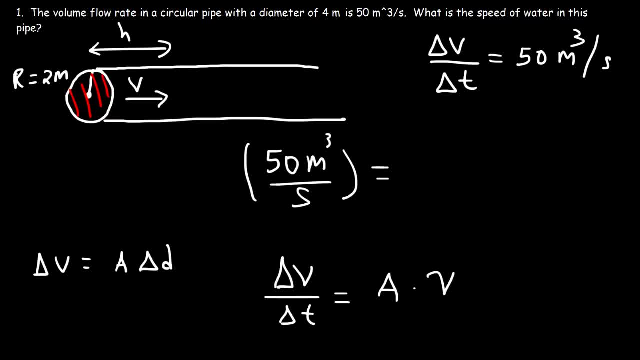 since we have a circle. So that's going to be pi times 2 squared and that's going to equal the speed. So we have 50 on the left, 4 on the right, 4 pi on the right, So it's 50 divided by 4 pi. 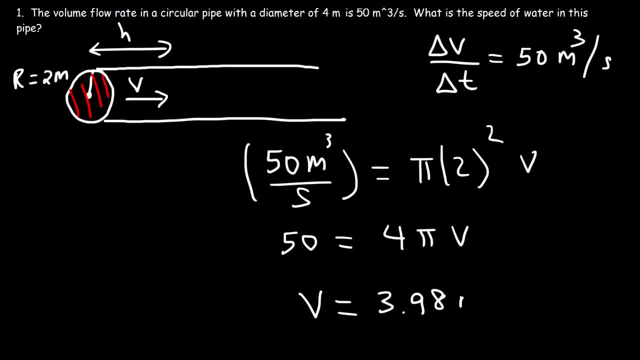 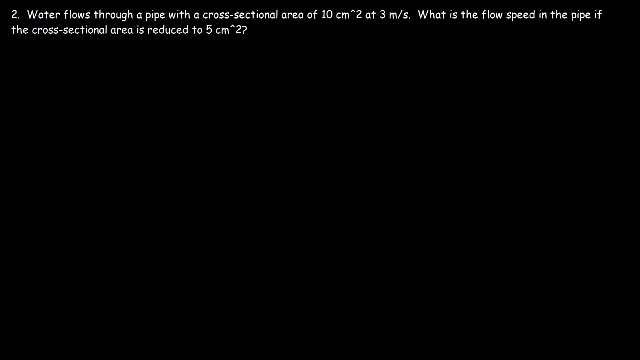 So the water is flowing at a speed of 3.98 meters per second, And so that's the answer to this problem. Number two: water flows through a pipe with a cross-sectional area of 10 square centimeters at 3 meters per second. 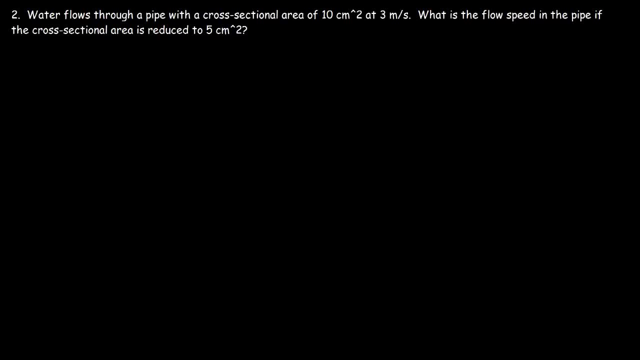 Number two. water flows through a pipe with a cross-sectional area of 10 square centimeters at 3 meters per second. what is the flow speed in a pipe if the cross-sectional area is reduced to five square centimeters? So, as always, let's draw a picture. 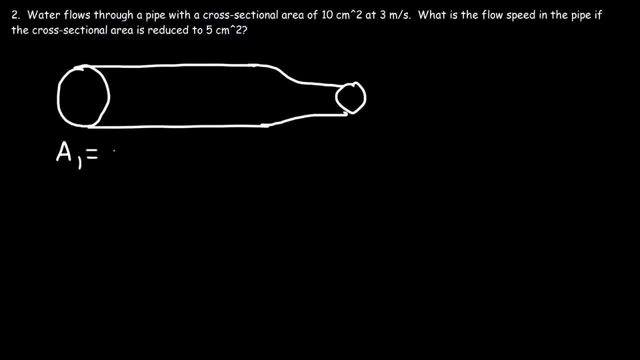 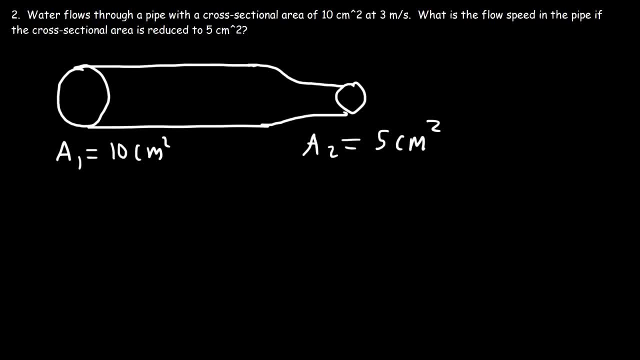 And on the right side, let's say a2.. that's five square centimeters. Now we have the speed of the water on the left. We need to find the speed on the right. On the left side the speed is three meters per second. So how fast should it be moving on the right side? So if the 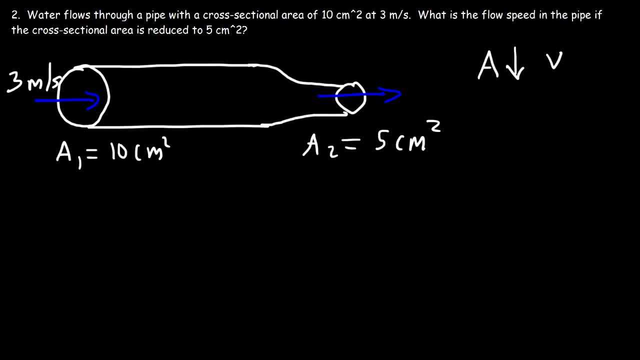 area decreases. what's going to happen to the speed? Now imagine if you have a water hose in your hand and water is coming out of it. What's going to happen if you place your thumb on the tip of the hose to partially block it? What's? 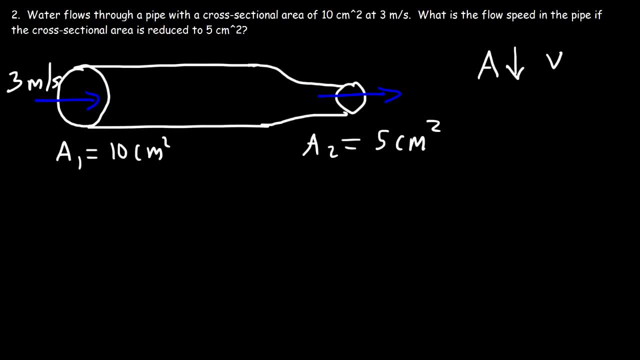 going to happen to the water coming out of the hose. If you partially block the opening of the hose, water is going to come out at a greater speed. Perhaps you've experienced that, And so anytime you decrease the cross-sectional area, the speed of the fluid is going to increase. Now how can we prove this with? 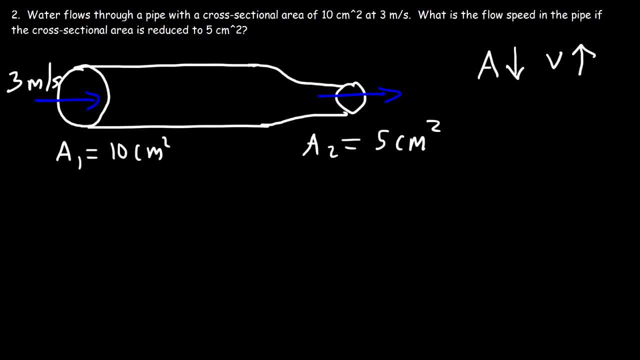 an equation. What we need to realize is that the mass flow rate has to be constant. The mass of water entering this container has to equal the mass of water leaving that container in a given time period. The mass flow rate is delta M divided by. 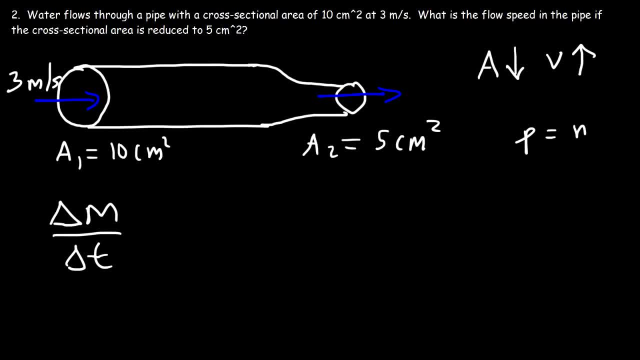 delta T And we know that density is mass over volume. so mass is density times volume. So delta M is going to be the density times. the change in volume And volume is area times height or area times displacement. So the change in volume is 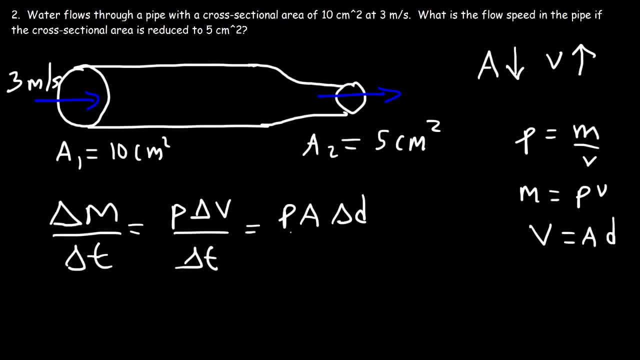 going to be the area times the change in height or the displacement, And displacement over time is velocity. So the mass flow rate on the left side is going to be the density of the fluid times. the area on the left side times the speed on the left side. And because 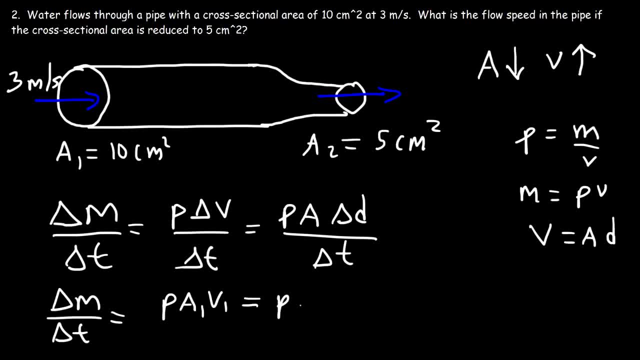 the mass flow rate is constant, that has to equal the density times the area on the right side, times the speed on the right side, And so we have the equation of continuity. Now, if the fluid is incompressible, which means that the 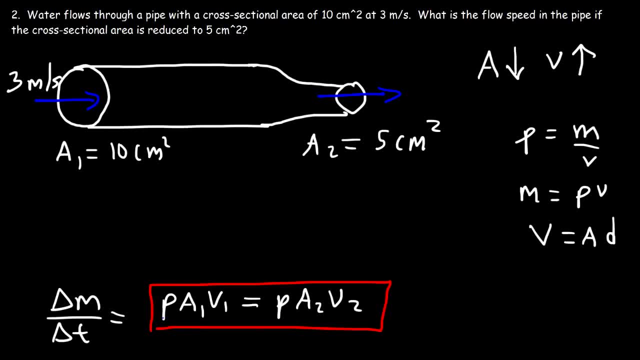 density of the fluid is constant, we can cancel the row. So for this particular problem, we can say that A1 times V1 is equal to A2 times V2.. Now A1 is 10 square centimeters. Now we don't need to convert the units to meters. 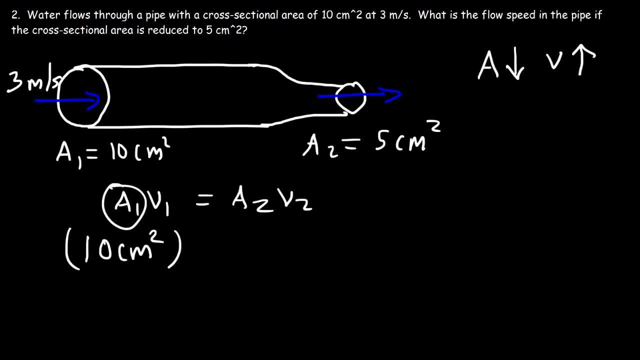 As long as A1 and A2 have the same units, it's going to work out fine. V1 is three meters per second, A2 is five square centimeters, And now we get to solve for V2.. So it's going to be 10 times 3 divided by 5. And so that's going to be. 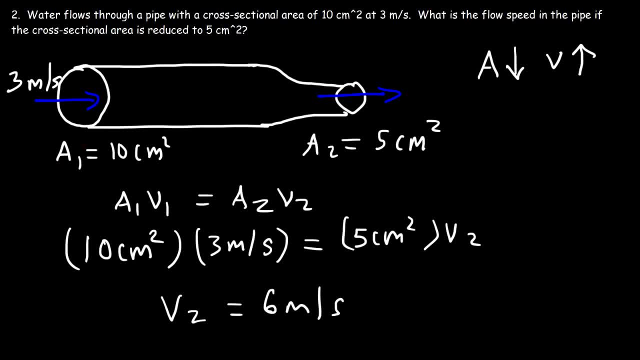 six centimeters. So notice what happened: We decrease the area by a factor of two, And so the velocity increased by a factor of two. It went from three to six. So as you decrease the cross sectional area, the flow speed is going to increase. 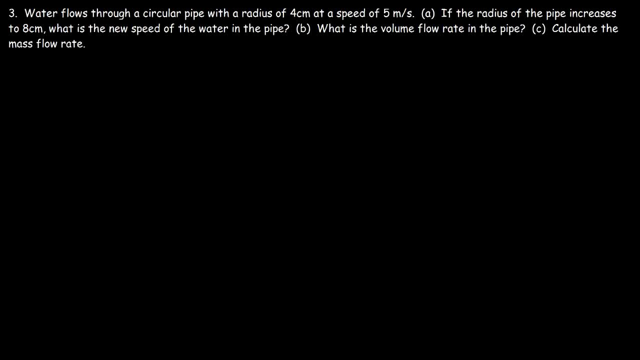 Number three: water flows through a circular pipe with a radius of four centimeters at a speed of five meters per second. If the radius of the pipe increases to eight centimeters, what is the new speed of the water in the pipe? So let's draw a picture. So that's the 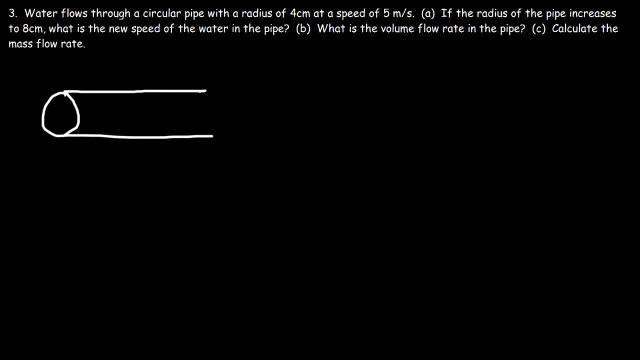 left side of the pipe, And it's going to get bigger this time. So on the left side, the radius is 4 centimeters. On the right side, the radius is 8 centimeters. So if we increase the radius of the pipe, what's going to happen to the speed? Well, 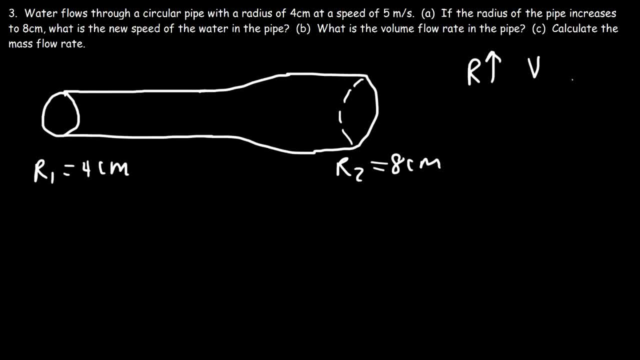 we've got our new pipe That's going to go from 10.. Hello everyone, Great, because it's wider. we know the speed is going to decrease, but we double the radius. so by what factor should the speed decrease? by two or four now? 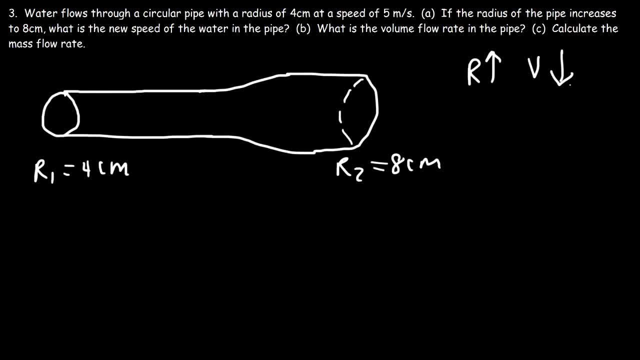 because the area is proportional to the square of the radius. the speed is inversely related to the square of the radius. so if we double the radius, 2 squared is 4, the speed should decrease by a factor 4, so it's going to be 5. 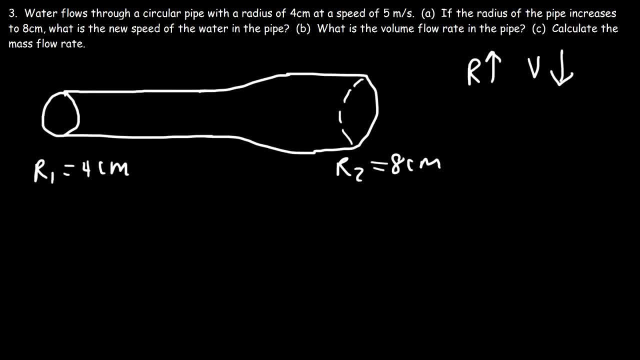 divided by 4, which is 1.25. but let's go ahead and prove that answer. so the speed is 5 on the left side and we need to calculate V 2. so we can use this equation: a 1 times V 1 is equal to a 2 times V 2. the cross-sectional area. 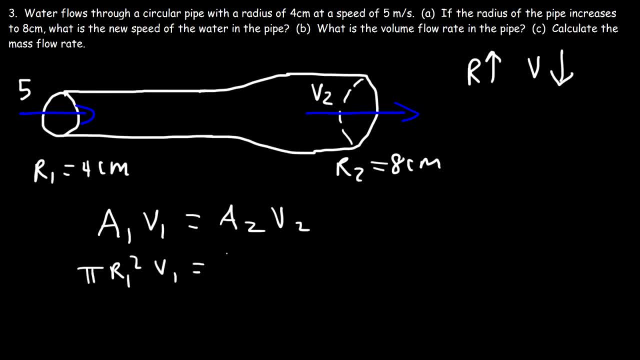 is PI R squared, so we can cancel PI in the equation. our one is 4, V 1 is 5. meters per second are two is eight and let's calculate V2. so it's going to be four squared times five divided by 8, actually divided by 8 squared. so four squared times five is 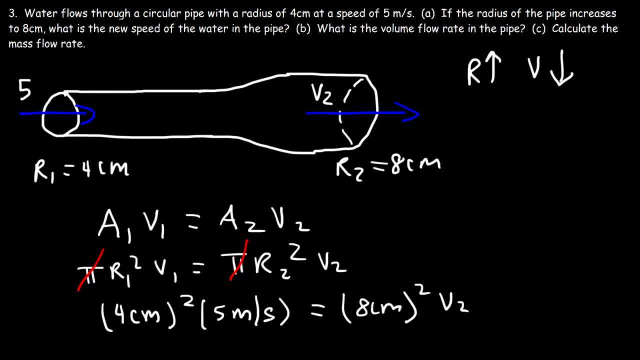 80 and 80 divided by 8 squared is 1.25. so that's the new speed. it's 1.25 meters per second. so if you double the cross-sectional radius, the speed is going to decrease by a factor four. if you triple the cross-sectional radius, the speed is going to decrease by a factor of three squared. 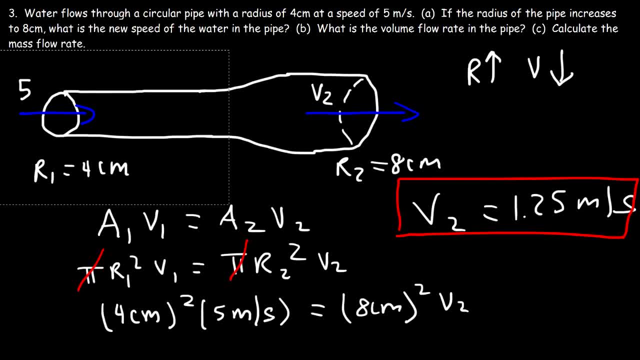 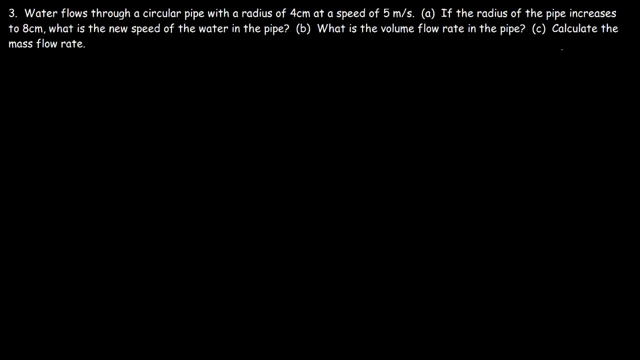 or nine. now let's move on to part b. what is the volume flow rate in the pipe? so, as mentioned before, volume flow rate is equal to the area times the velocity. so on the left side the area is going to be pi r squared. so if we use the right side value, 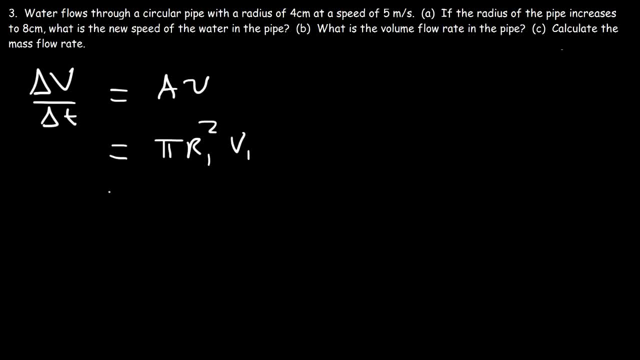 pi r2 squared times v2, it should give us the same answer. so on the left side the radius is four centimeters, but we need to convert that to meters this time. so four centimeters is 0.04 meters and the speed is five meters per second. 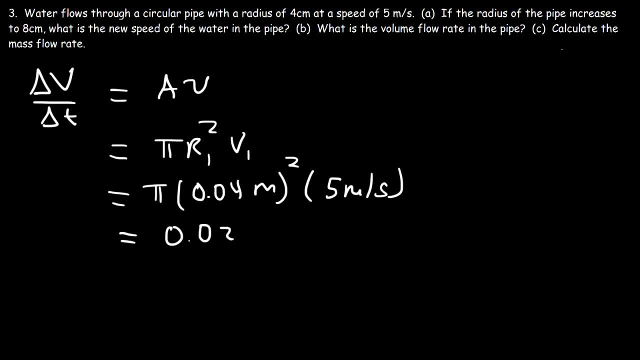 and so the volume flow rate is 0.0251 cubic meters per second. now, if you use the values for the right side of the pipe, you should get the same answer. so it's going to be pi r2 squared times v2. so r2 in this case is going to be 0.08 and v2 is 1.25. 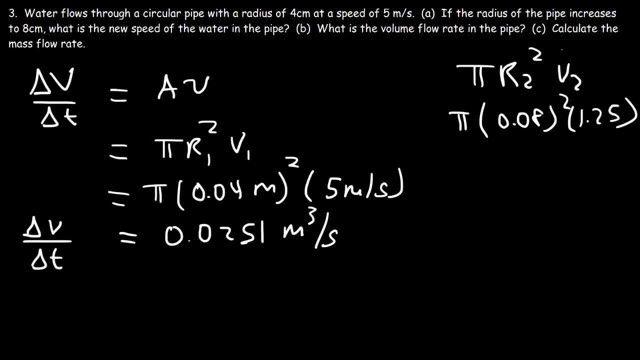 and this will give you the same answer of point 0251 cubic meters per second. so this will give you the same answer of 0.0251 cubic meters per second, and this will give you the same answer of point 0251 cubic meters per second. 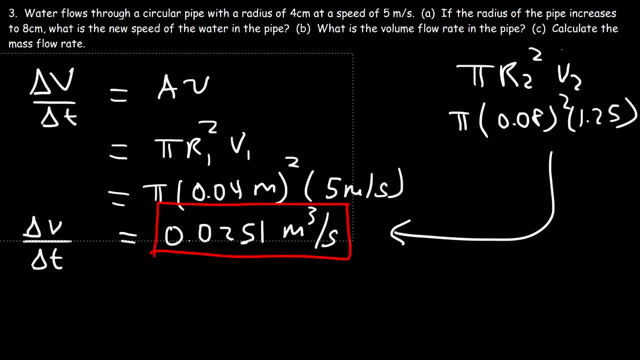 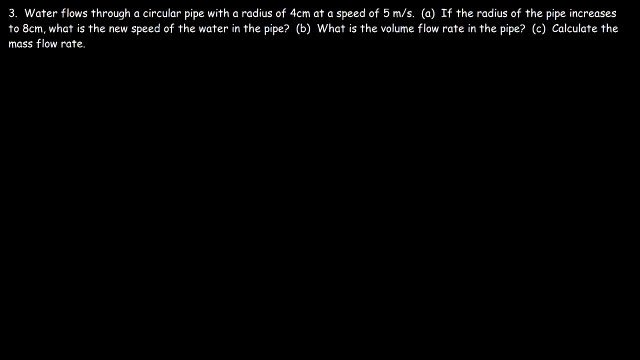 Now let's move on to part C: Calculate the mass flow rate. The mass flow rate is equal to the density of the fluid, times the cross sectional area, times the speed. So let's focus on the values. on the left side. The density of water is 1000 kilograms per cubic meter. 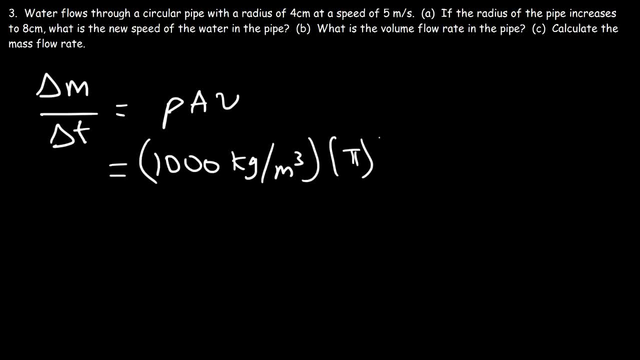 The cross sectional area is pi r squared, so that's pi times the square of the radius, which in meters is 0.04.. You just gotta divide that by 100.. And the speed on the left side is 5 meters per second. 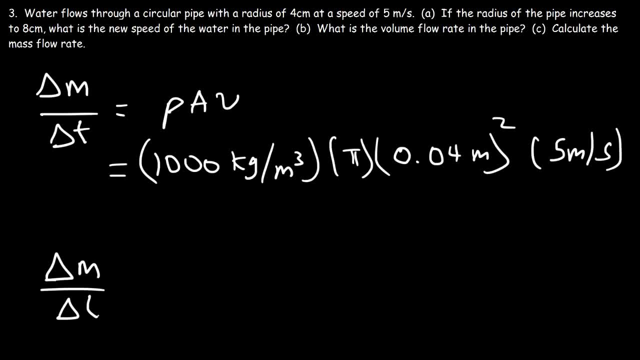 So basically, the mass flow rate is simply the density of the fluid times the volume flow rate. A times V represents the mass flow rate. A times V represents the volume flow rate. So pi times 0.04, squared times 5, which is this portion right here that gave us a volume. 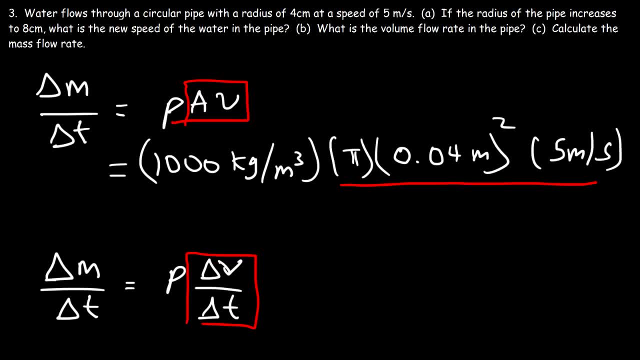 flow rate of 0.0251.. Then if we multiply that by the density of the fluid, that's going to give us the mass flow rate, which is 25.1 kilograms per second. So now you know the relationship between the mass flow rate and the density of the fluid. 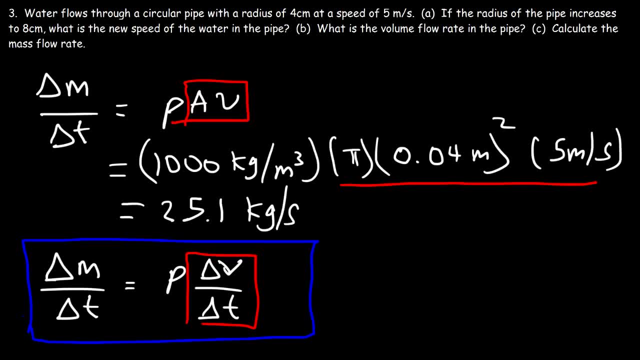 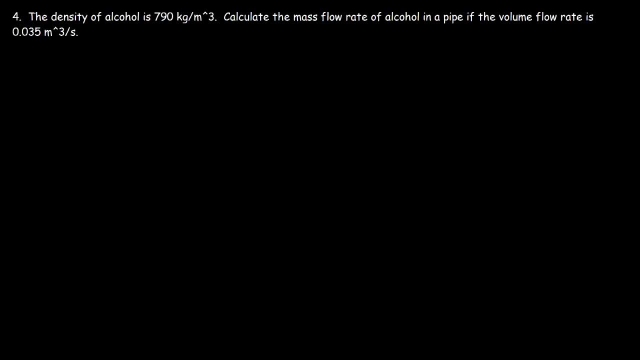 So let's move on to part C: Calculate the mass flow rate. The mass flow rate is simply the density times the volume flow rate. So this is the answer to part C. So here's the last problem in the video. So we're given the density of alcohol. 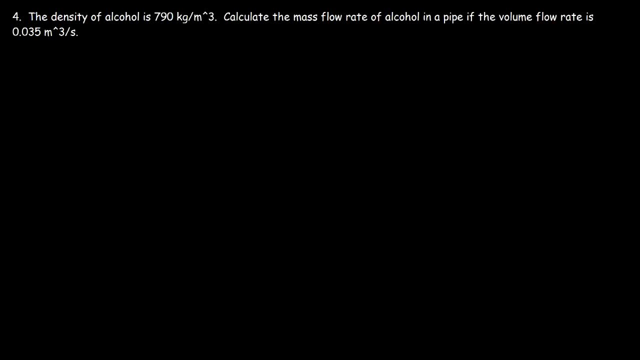 And our goal is to calculate the mass flow rate of alcohol in a pipe, given the volume flow rate. So, as mentioned before, the mass flow rate is simply the product of the density times the volume flow rate, And it makes sense because mass is density times volume. 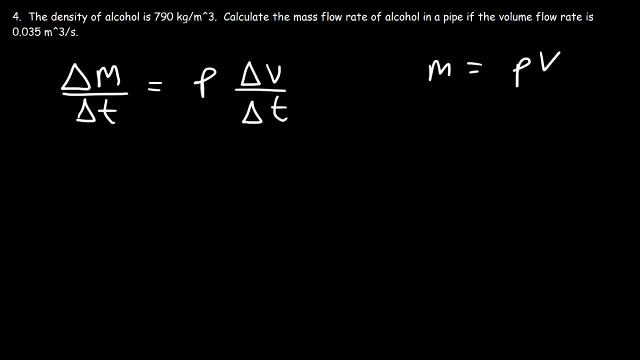 So the mass flow rate is going to be the density times the volume flow rate. So the density of the alcohol is 790 kilograms per cubic meter And the volume flow rate is .035 cubic meters per second. So we can see the unit cubic meters will cancel.